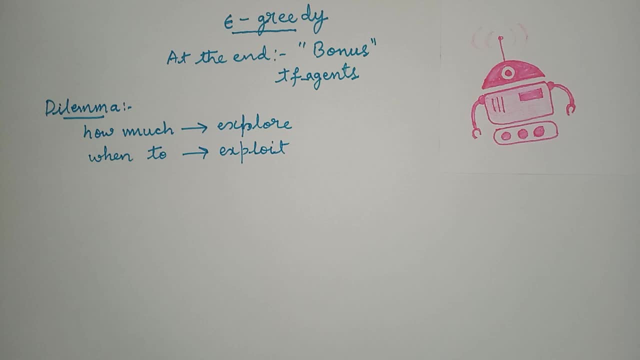 Exploiting, you may regret the possibility of getting higher reward in the future. So in order to maximize the reward, You need to balance between exploration and exploitation. There are many different methods and strategies to balance between exploration and exploitation. Some of the examples are: Epsilon- greedy method. 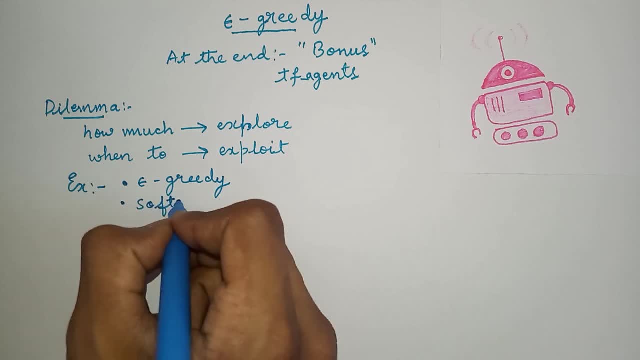 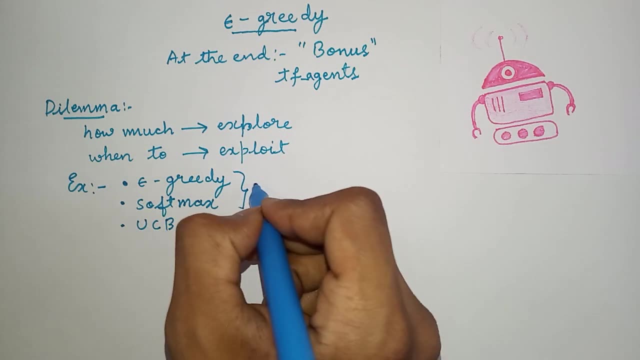 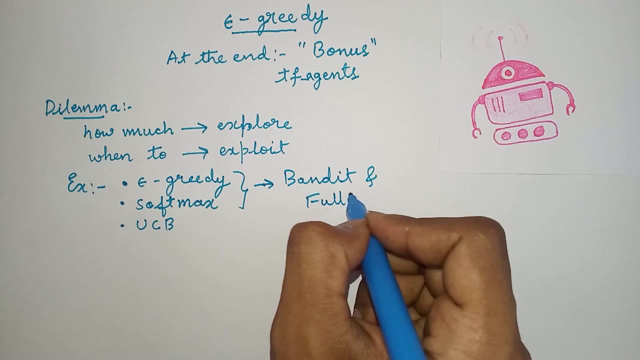 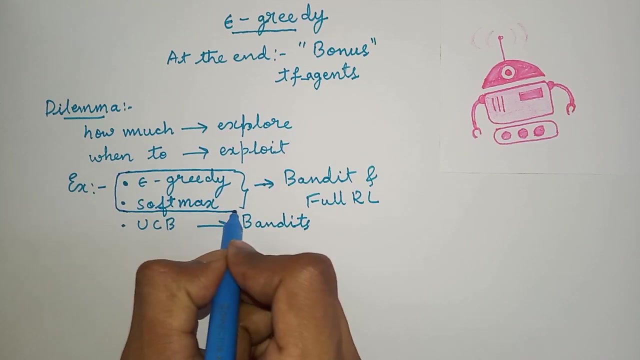 Softmax method, UCB, UCB- upper confidence bonds. These two methods are used in both bandits and Full RL problem, and this is used more specifically for bandits. Before going to Epsilon greedy method, Let me talk about action values. What are action values? action values are represented by Q of A. 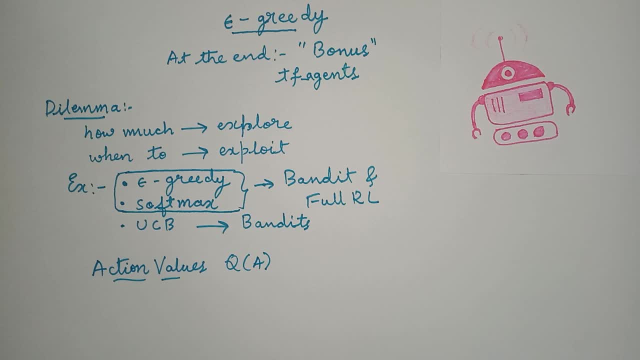 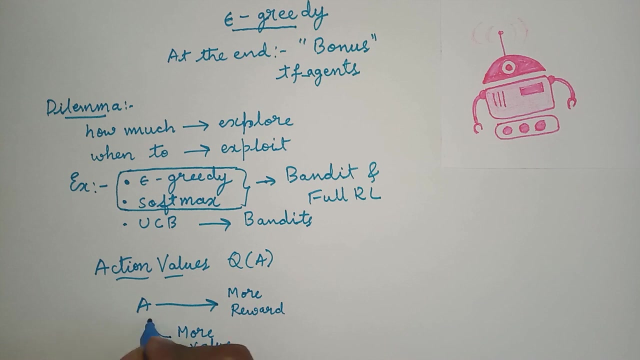 In RL during learning process, we calculate the value of each action and the action gives more reward gets more value. we assign more value to the action that gives more reward. similarly, if an action a, a, 2, let's take it as a 1 and a. 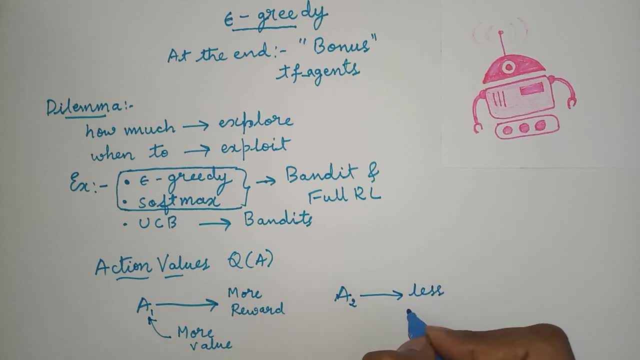 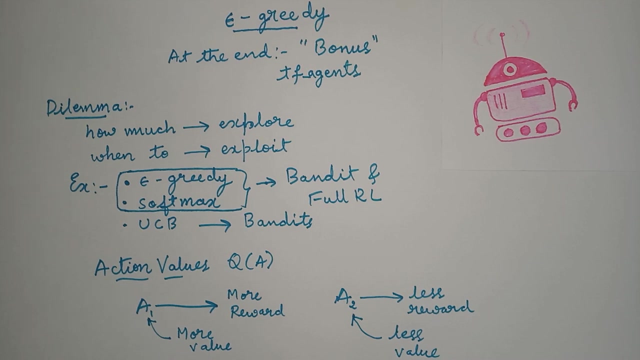 2 gives less reward. we give less value. there are different methods for calculating in action values. all these methods are known as action value methods. we call them as action value methods. there are different action value methods and one of the basic and most popularly used action. 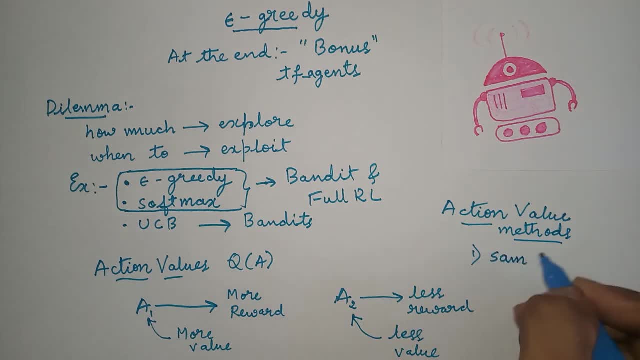 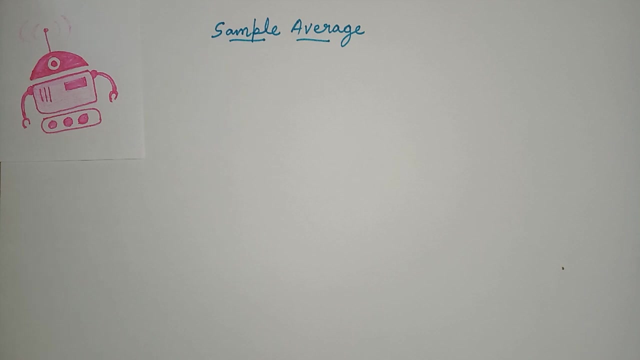 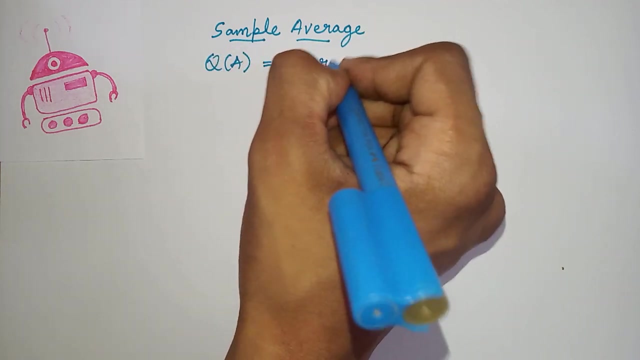 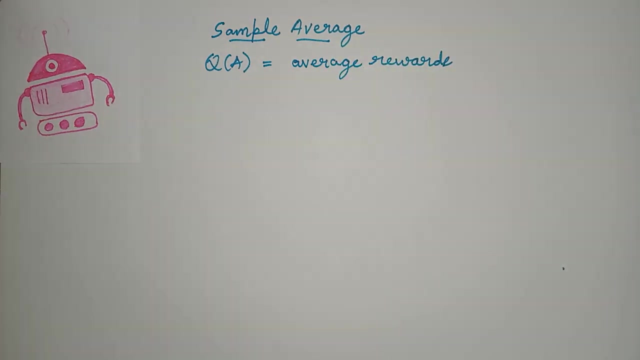 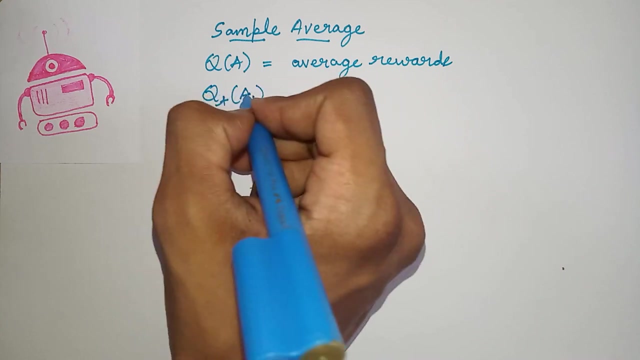 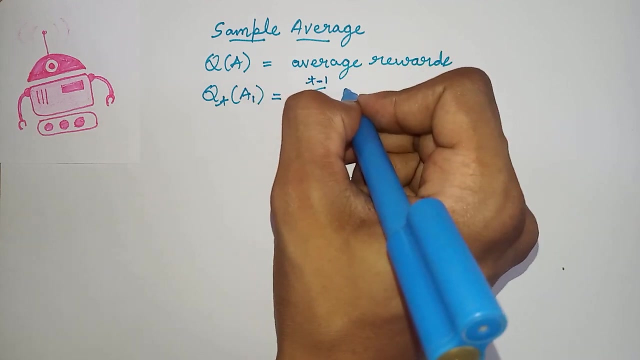 value method is sample average. sample average method. in sample average method the action values Q of a are nothing but average. rewards action value at any time: step t action value of a1 at any time time step t is given 1 by summation of i is equal to 1 to t minus 1 reward into this is an indicator function. 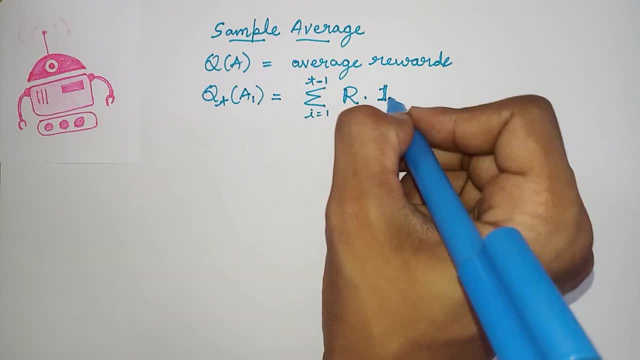 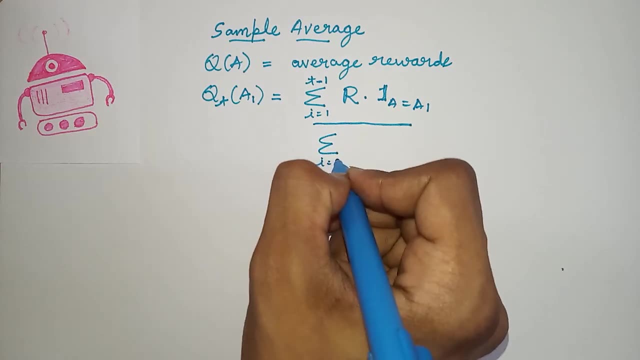 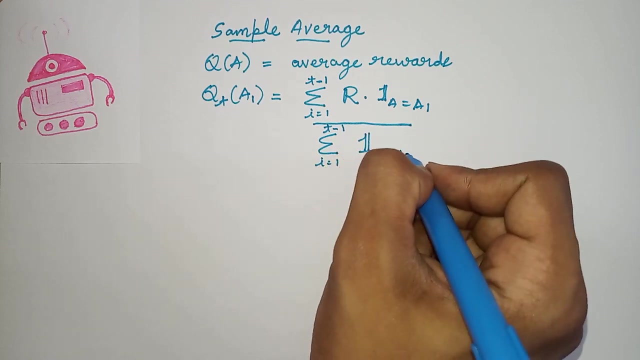 and this function is 1. whenever an action is a 1, a is equal to a 1, divided by summation of i is equal to 1. to t minus 1. indicator function a is equal to a 1 and the greedy action is given by: 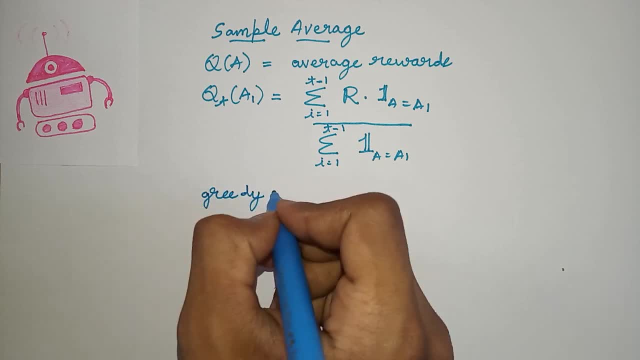 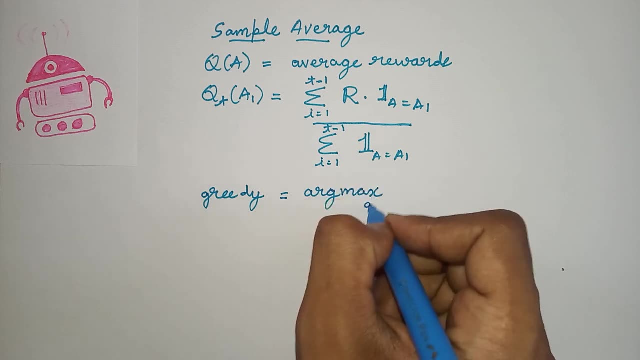 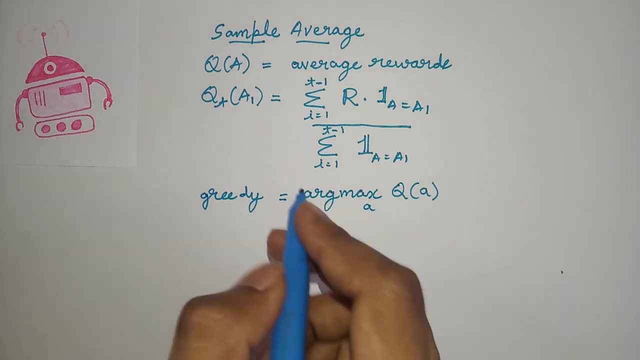 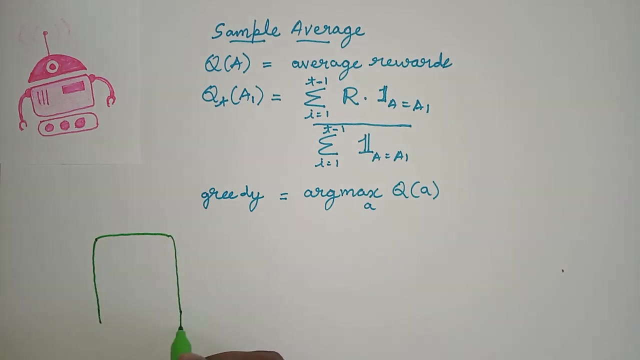 greedy action is given by argument: max of a, q of a. this is a greedy action which is nothing but maximum action value among all the different actions. let me take an example of a k-arm bandit. bandit is nothing but a slot machine and this slot machine has got liver in k-arm. 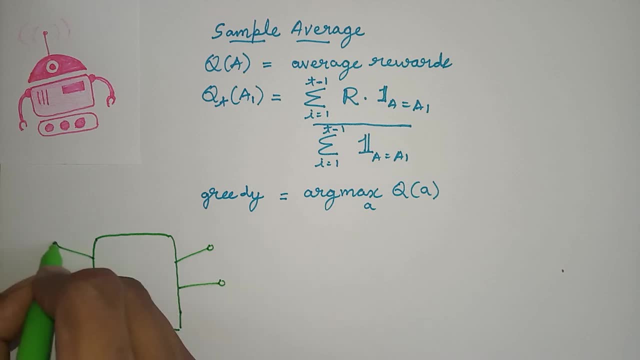 bandit, there are k livers. let me take an example of 5-arm bandits. and this is a screen and there is some output in the screen- star or moon- and these 3 signals will give aство and star. let us consider the action of. 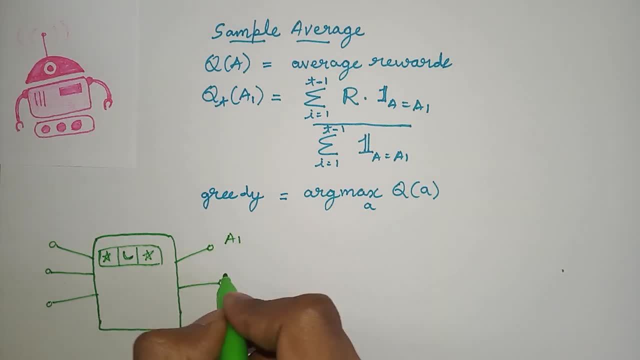 and star. let us consider the action of pulling this arm as a 1 and this similarly a 2, a 3, a 4 and a 5. let us similarly a 2, a 3, a 4 and a 5. let us calculate the action values at any time. 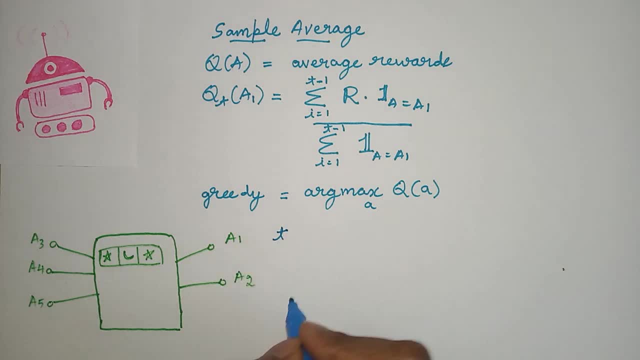 so if t, let us use sample average method. so if t, let us use sample average method for calculating an action value at any. for calculating an action value at any, all these actions be: Qt of a1 is equal to 4, Qt of a2 is equal to 3, Qt of a3 is: 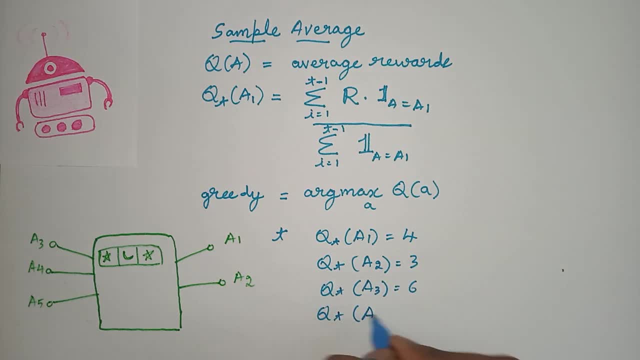 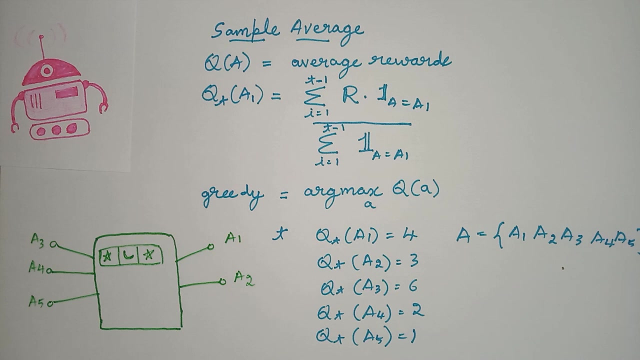 equal to 6,. Qt of a4 is equal to 2,. Qt of a5 is equal to 1.. Let a be the set of actions. a is equal to a1,, a2,, a3,, a4 and a5.. In this example, greedy action is. 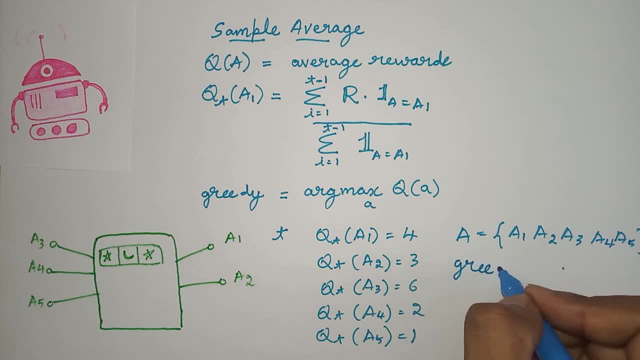 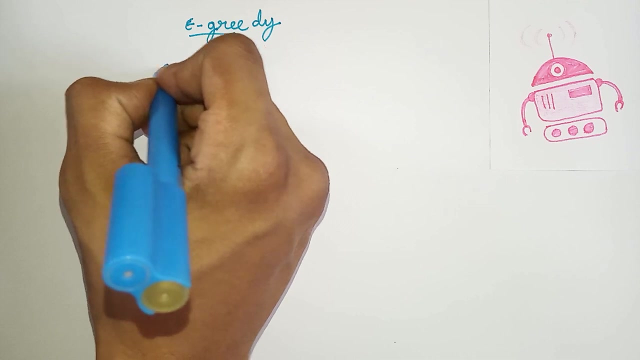 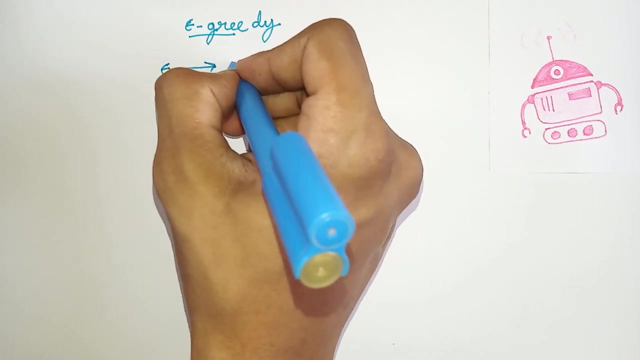 given by greedy action is equal to find the highest among these six Greedy action is given by. greedy action is a3.. Now let us jump to the epsilon greedy method. In epsilon greedy method, with probability of, with a small probability of epsilon, we picked action at uniform. 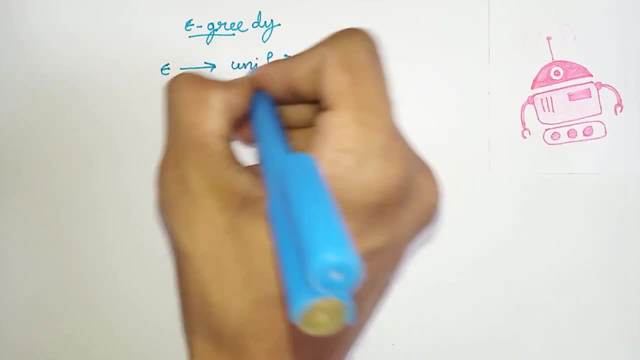 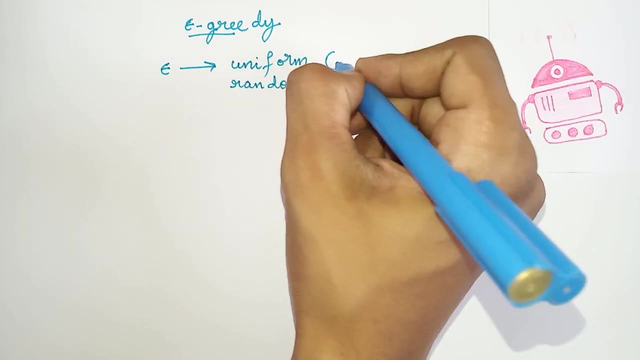 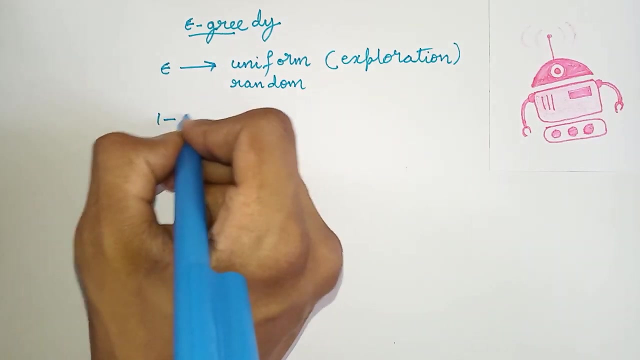 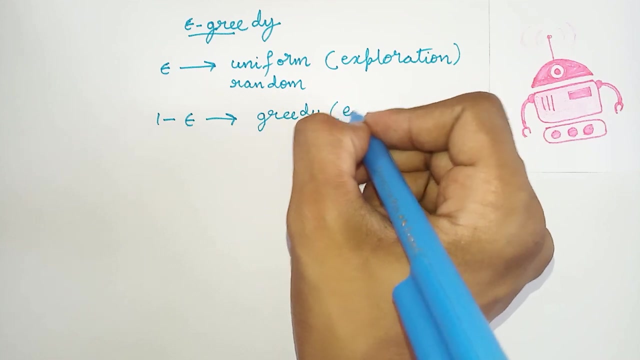 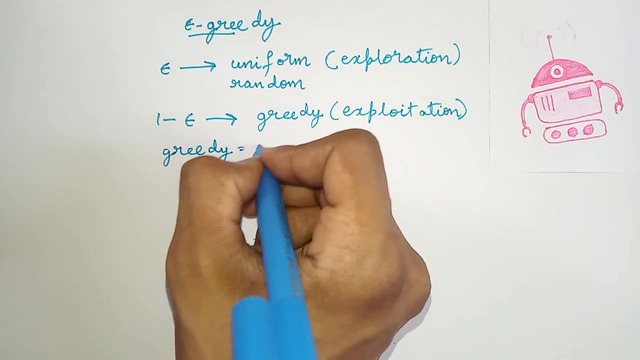 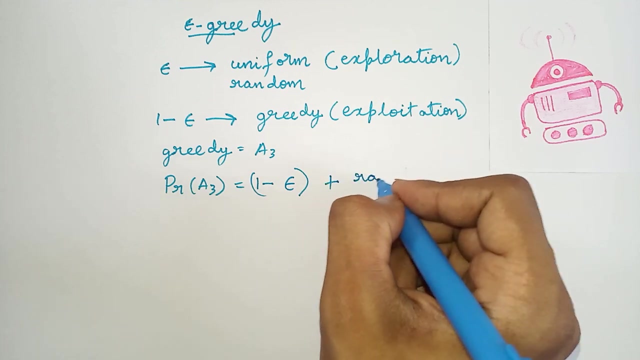 random. This corresponds to exploration- And with the probability of one, one minus epsilon, we pick a greedy action. Nothing but exploit. In our bandit example, the greedy action is given by a3. Greedy what a3.. So probability of choosing a3 is equal to 1 minus epsilon, plus random pick, Because 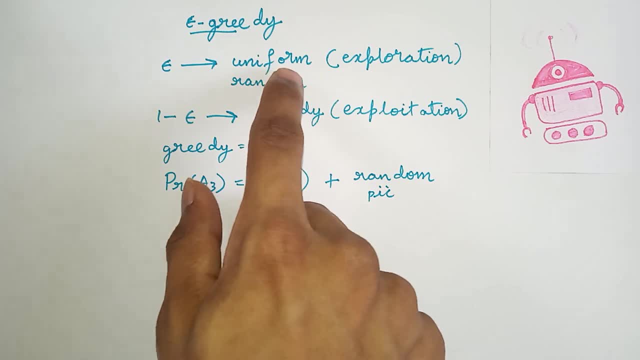 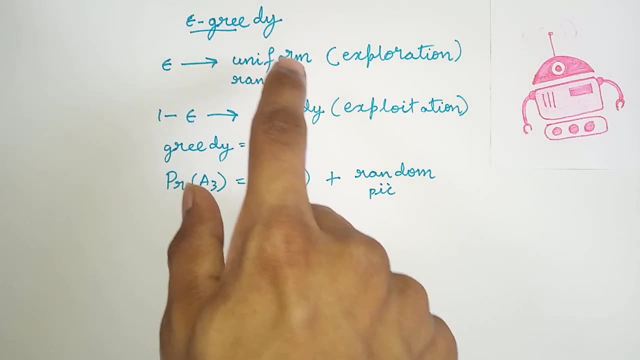 even during random action selecting an action at uniform random, we can also pick a3, that is an greedy action. Greedy action is also applicable for picking an action at random, So that small probability is given by random pick and with the probability of 1 minus epsilon. 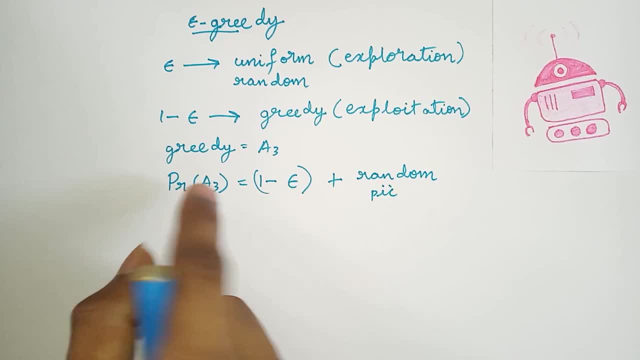 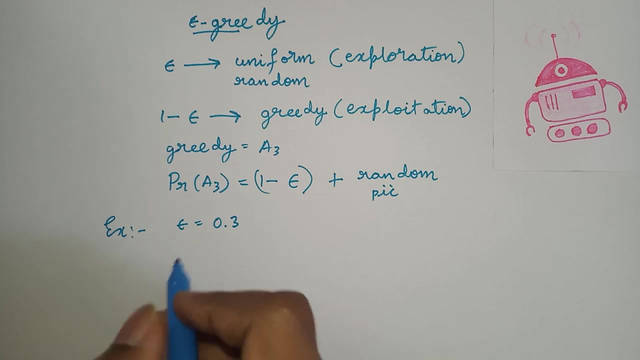 plus, with small probability, we pick a greedy action. Let's take an example. Let us consider the value of epsilon be 0.3.. For our bandit example, the probability of choosing action a3 is 0.7,, that is, 1 minus 0.3 is 0.7.. So for every 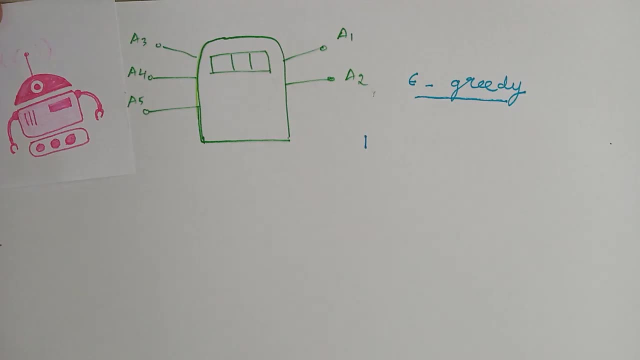 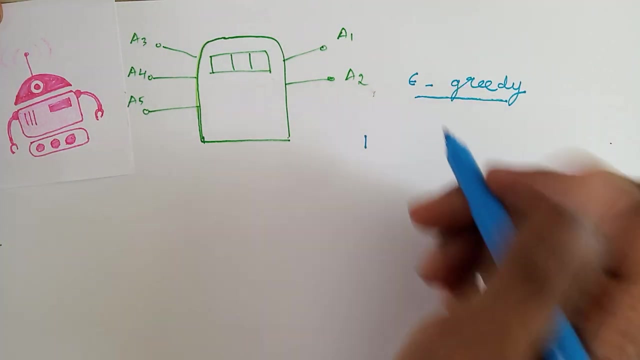 7 in 10 action we take now let me consider a same bandit example. If we apply epsilon greedy method for exploration and exploitation, with the probability of 1 minus epsilon, we choose greedy action, That is, action a3. And with the probability of epsilon, we choose either action a1, a2,. 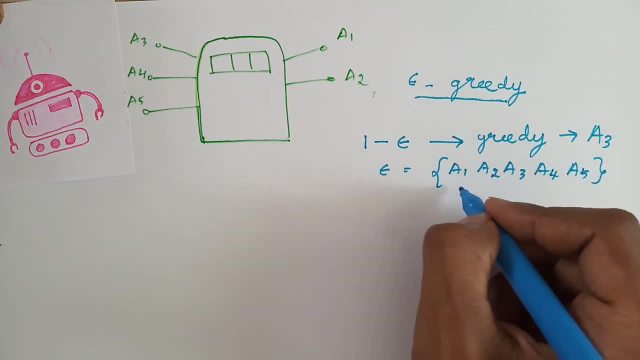 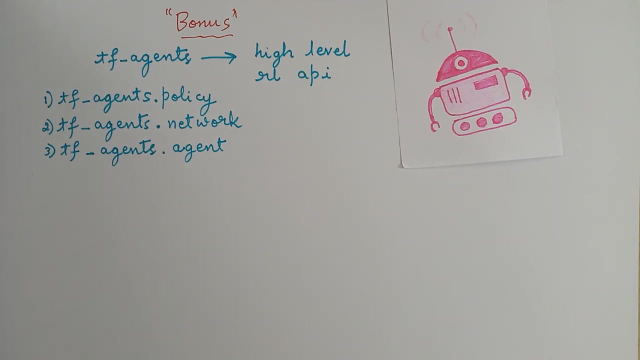 a3, a4 or a5 randomly at uniform, Uniformly at random. So this is the probability of decision of taking action a3 as 0.3.. Now it's time for bonus. As you know, tfAgent is a high-level RL API from Google TensorFlow. 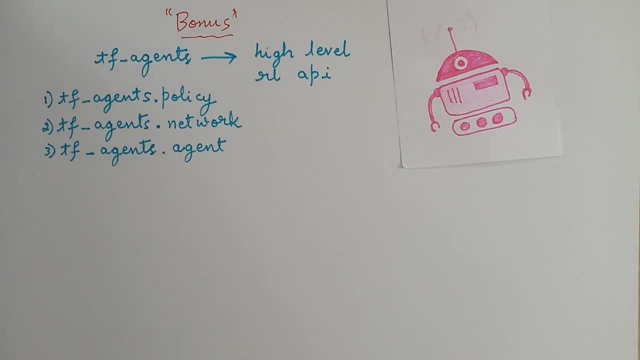 that is used to implement reinforcement learning, And these are the very common packages that we use to implement reinforcement learning in tfAgent. tfAGentpolicy contains different policies. tfAGentnetwork is used to build different types of network, And tfAGentagent. 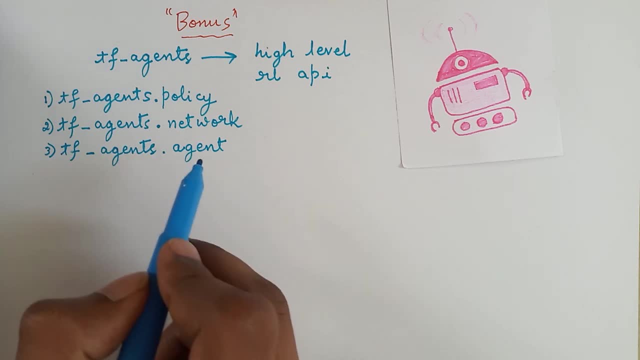 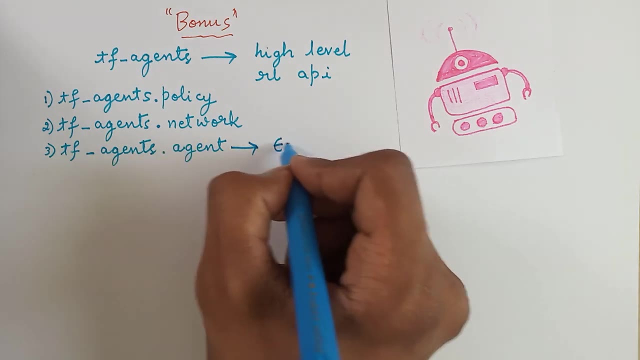 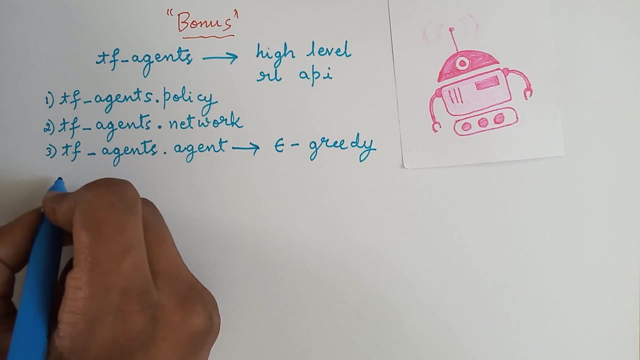 is used to build different types of data. tfAGentnetwork is used to build different is used to configure a reinforcement learning agent. Here, while building this reinforcement learning agent, we need to specify epsilon greedy. Let me take an example of building a DQN agent.